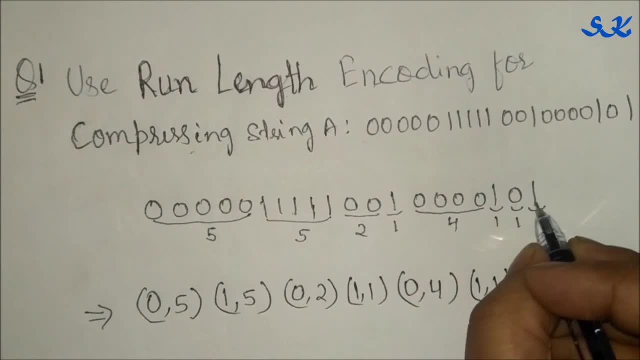 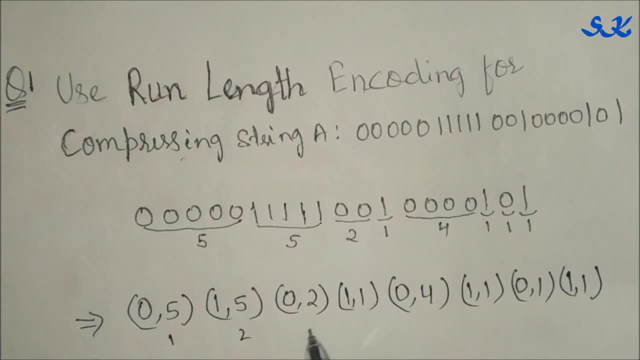 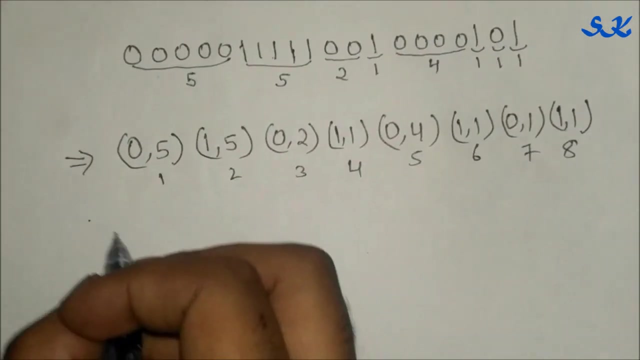 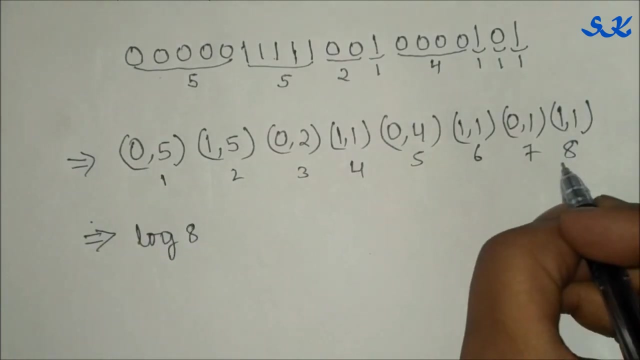 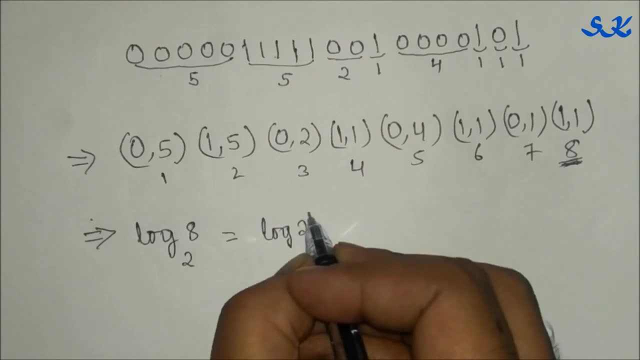 is one time, again one is one time. now. count the term this: one, two, three, four, five, six, seven, eight. so now the third step is. third step is we find the value log. we write eight here because the total term is eight, eight, two, so log two to the power two, two, so three log. 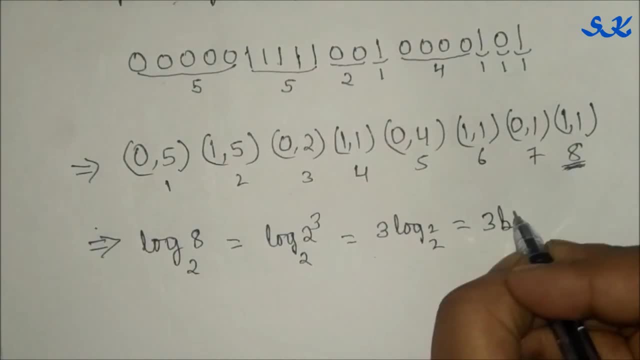 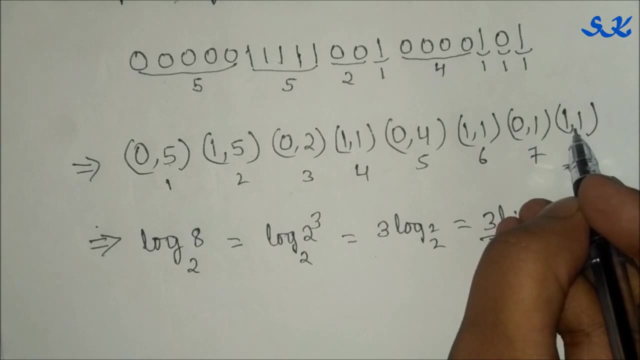 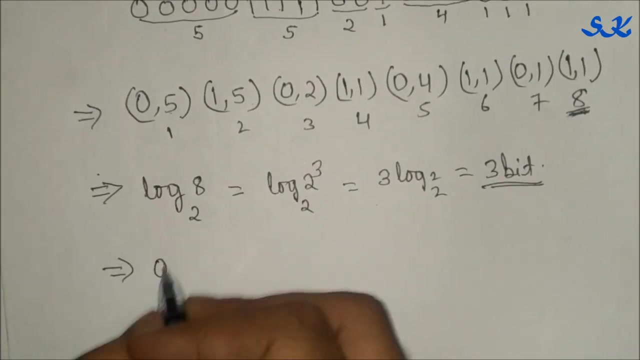 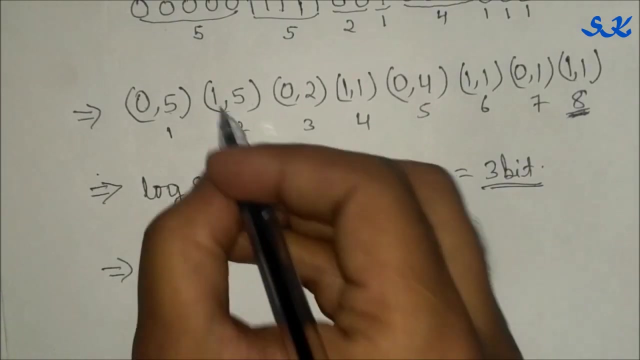 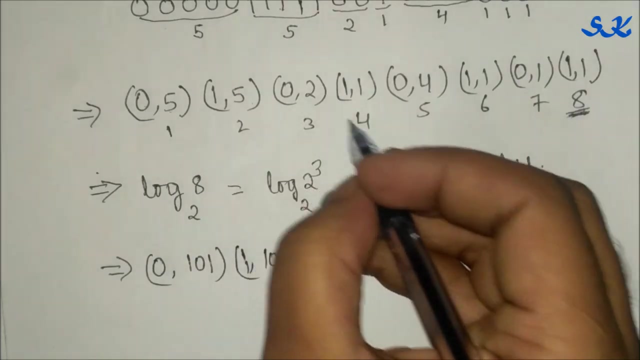 two, two, so three, three bit. so we take three bit for this term: five, five, two, one, four, one, one, one. so next step is zero and we can write five s, one zero, one in three bit and again one, five s one zero, one in three bit and again zero two. we write two in three bits. so zero, one, zero. 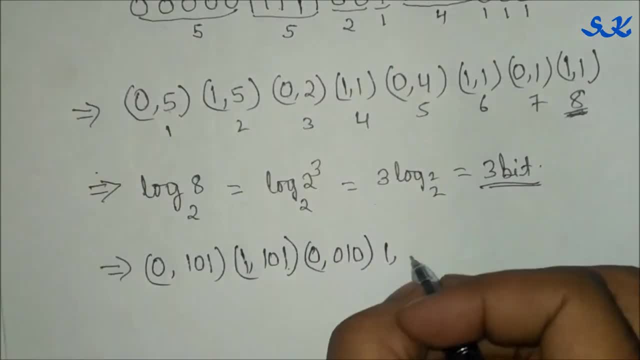 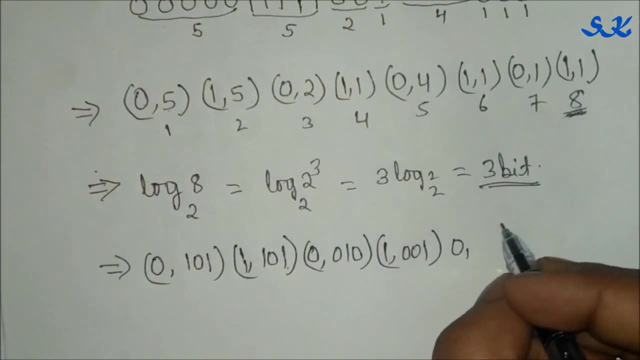 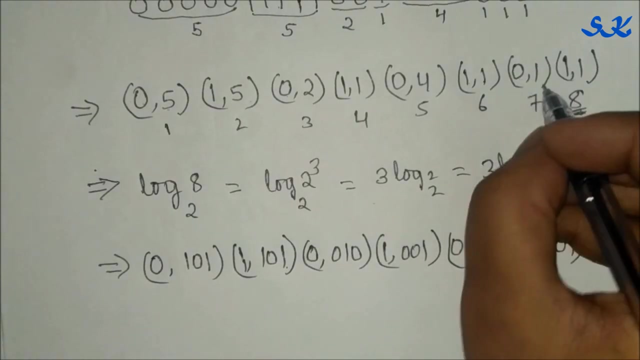 and again one. we write one in three bits, so zero, zero, one, zero. we write four in three bit, so one, zero, zero. and again we write one in one in three bit: one, zero, zero, one. and again we write, uh, one in three bit, so zero, zero, zero, one.